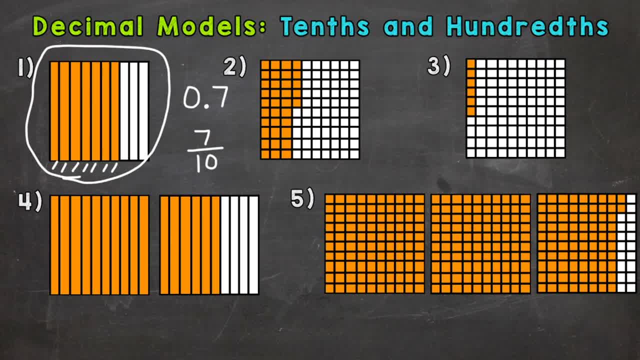 Each column has ten hundredths. We don't need to count each individual piece, So we can go 10, 20, 30 and then count the individuals. So 31, 32, 33, 34, 35 hundredths, And we would write it as: 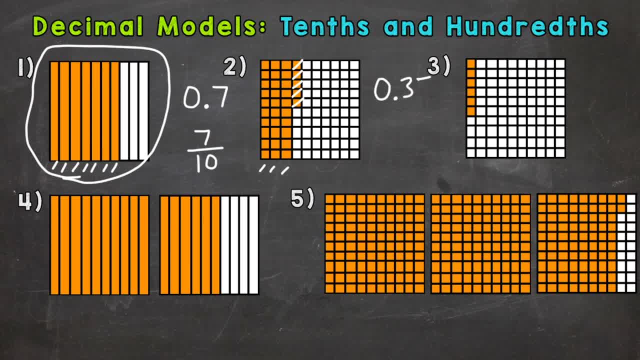 zero holes. decimal: 35 hundredths. Or, in fractional form, 35 over 100, 35 hundredths. So on to number three, where again we're going to be working with hundredths. Now, this time we don't have any full columns, So we can just count the. 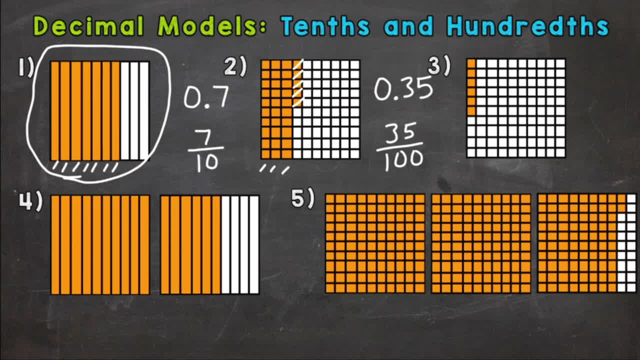 individual hundredths, And for number three we have one, two, three, four, five, six hundredths. A very common mistake would be writing it as zero holes decimal and then a six in the tenths place, So that represents six tenths. We don't want six. 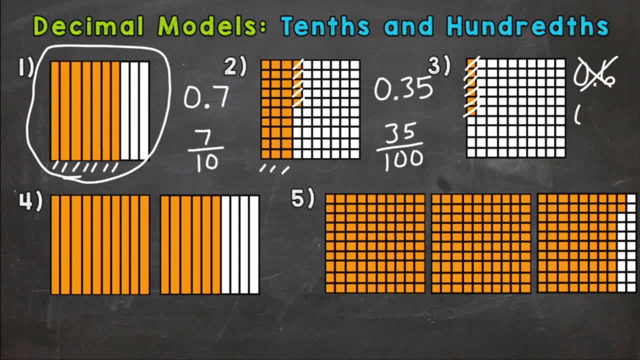 tenths. We want six hundredths. So we need zero decimal, a zero in the tenths, to push that six over to the hundredths place. So six hundredths, or in fractional form, six over one hundred. Now numbers four and five we're going to. 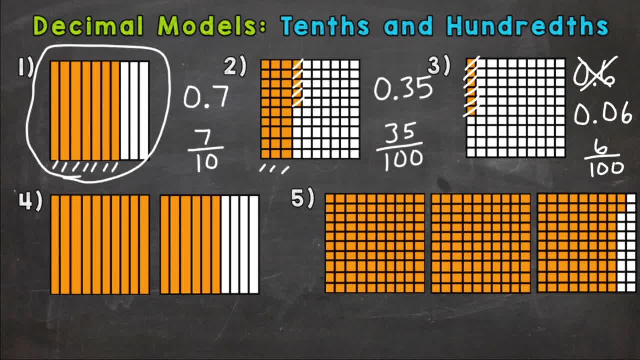 involve whole numbers here. Number four: we have one full square filled in here, so that represents one whole. And then our second square. we don't have the full square filled in, so that's where our decimal or fraction comes into play. 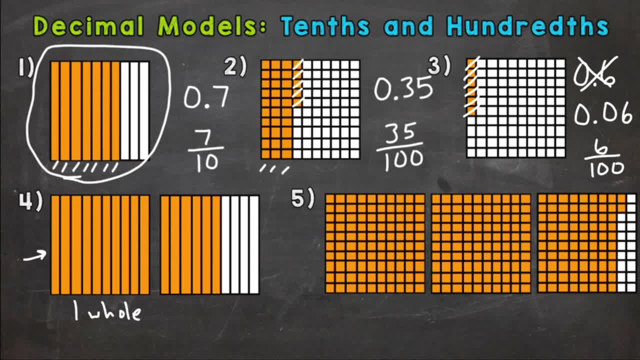 So this is going to be tenths. Let's see how many tenths we have filled in: One, two, three, four, five, six. So we need to write out one and six tenths and it's going to look like this: 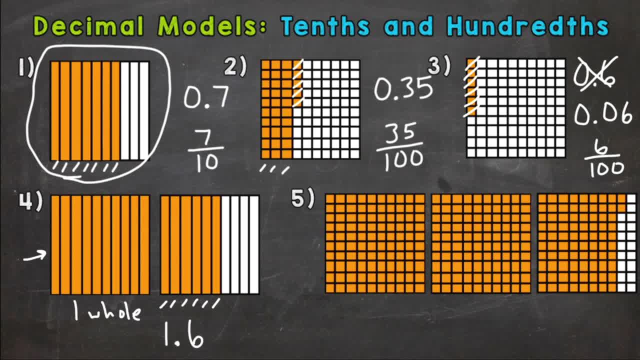 One and six tenths, Or in fractional form, one and six tenths, On to number five here, where we have two full squares filled in. So this is one whole and then two wholes. Now, as far as the decimal or fractional square, here we can start by counting by tens, because